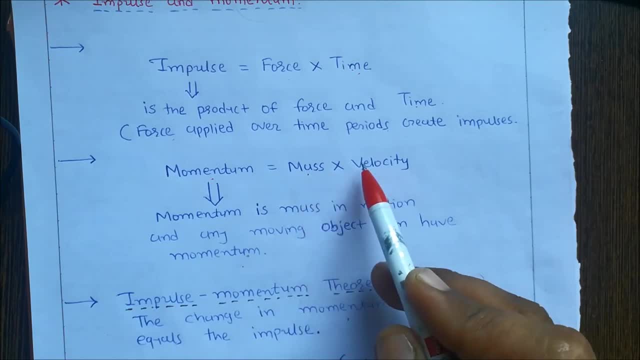 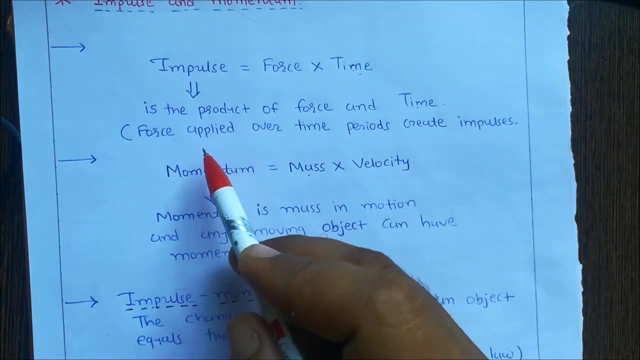 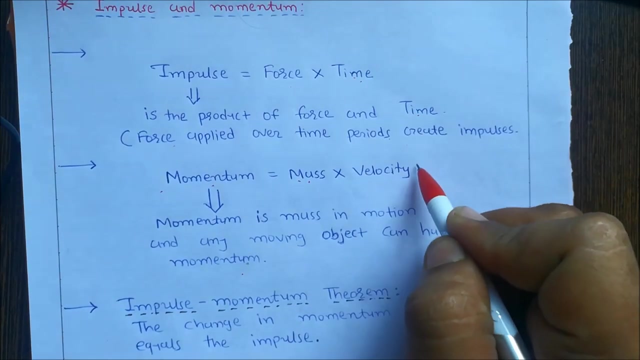 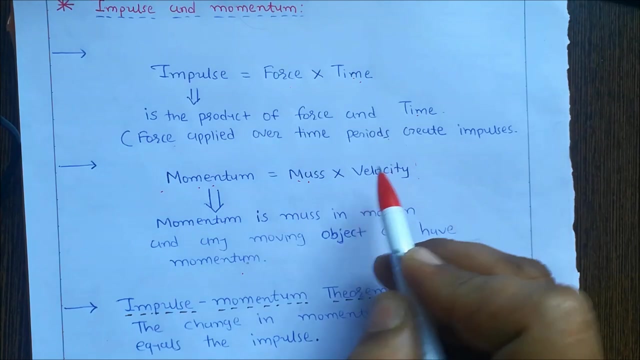 of momentum. So momentum is the product of mass and velocity. An object that is not moving has zero momentum. Momentum is a measure of how difficult it is to stop of an object. A slow moving large object has a large momentum and a fast moving small object. 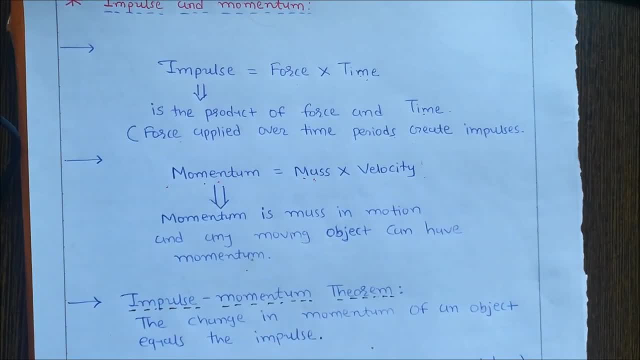 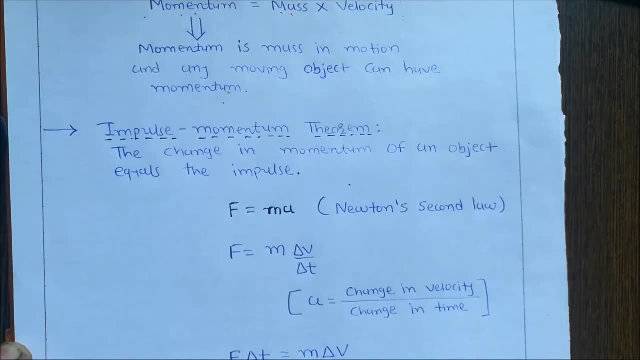 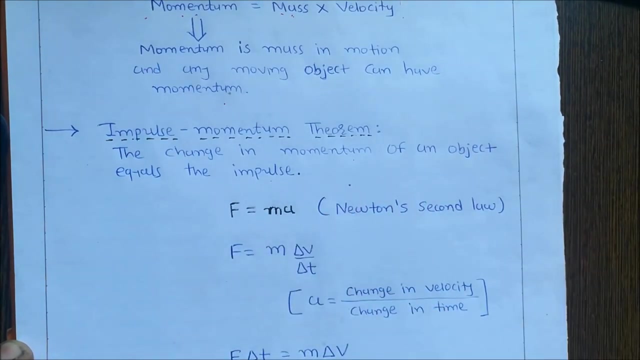 also has a large momentum. So momentum is basically mass in motion and any moving object can have momentum. So what is the basic relation between impulse and momentum? So impulse-momentum theorem states that the change in momentum of an object equals the impulse. So how we derive this? 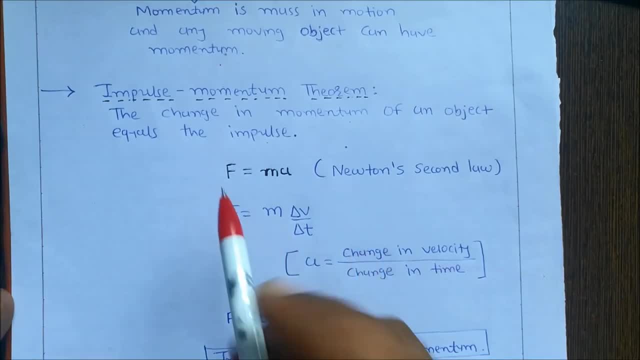 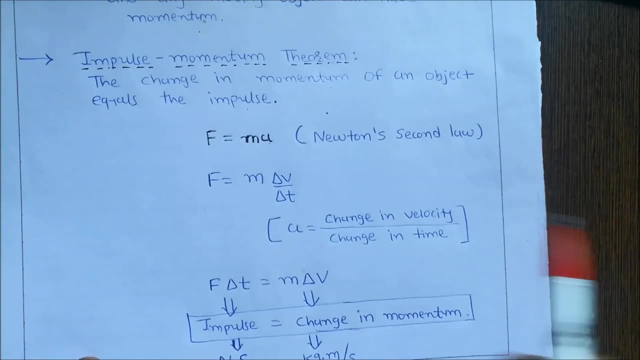 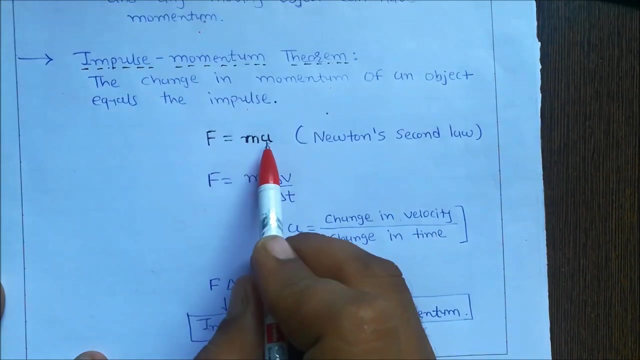 relation. So according to Newton's second law of motion, we can write: F is equal to m. And what is the basic definition of acceleration? So acceleration is equal to change in velocity divided by change in time. So in place of acceleration we can write delta v by delta t, So f is equal. 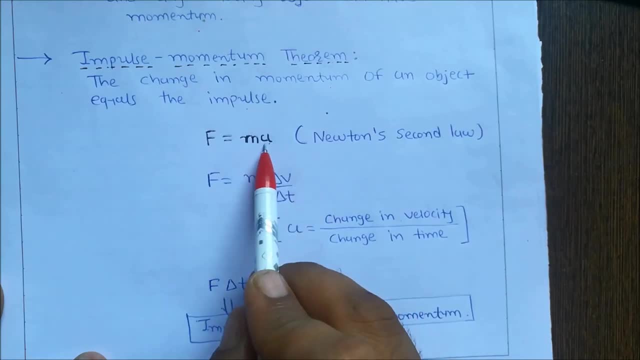 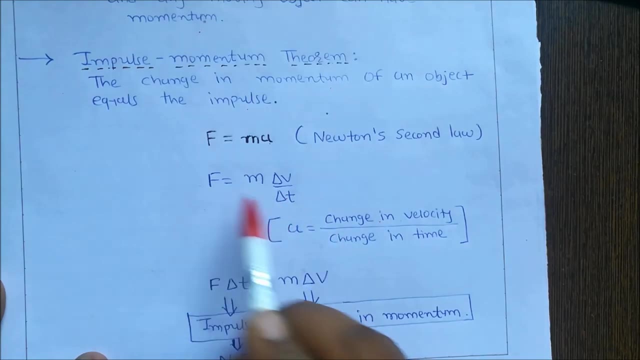 to m, delta v by delta t, because acceleration, that is change in velocity divided by change in time. So rearrange this equation. So f into delta t is equal to m into delta v. So we know that force multiplied time, that is, impulse and mass multiplied change in velocity. 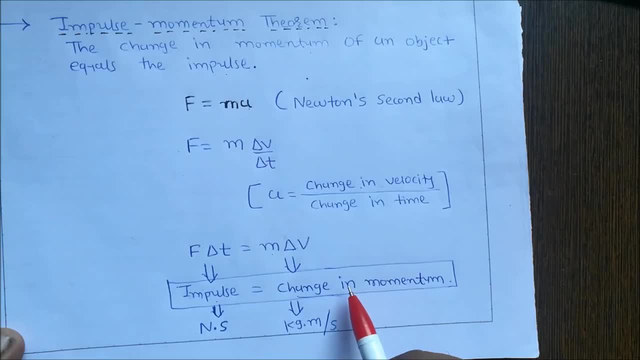 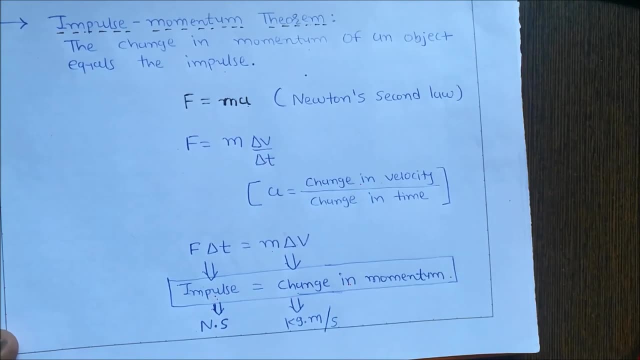 that is change in momentum. So we can say that the change in momentum of an object equals the impulse. So what is the unit of impulse? So here, force unit, that is Newton, and time that is second. So impulse unit, that is Newton, into second, And here, momentum, unit which? 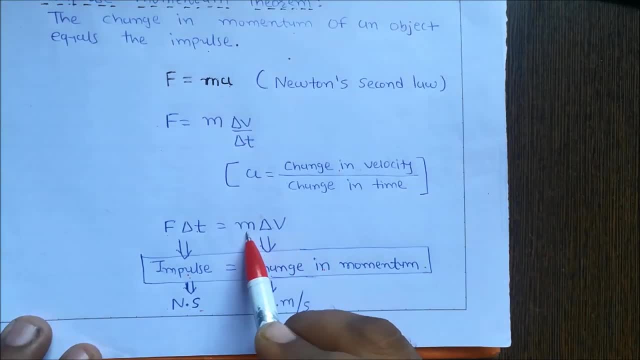 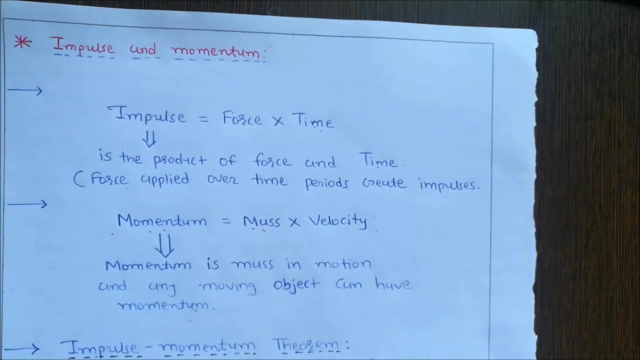 or you can say: change in momentum unit, that is kg, into meter per second. So because mass unit, that is kilogram, and velocity, that means meter per second. So kg into meter per second. Again, I repeat: impulse means force multiplied time, Or you can say that a very large force.